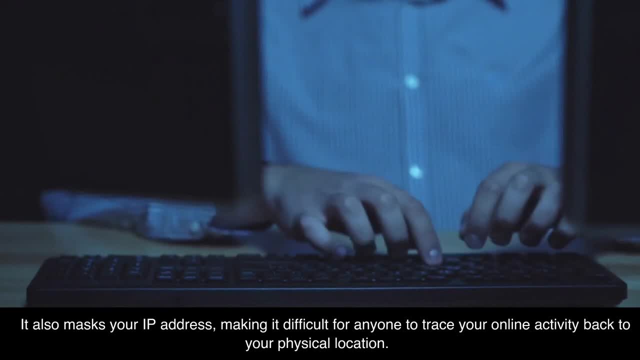 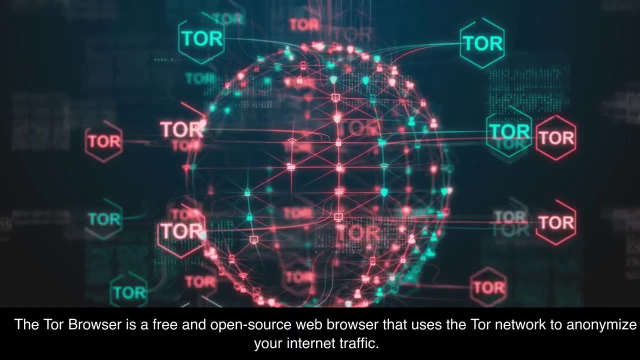 making it difficult for anyone to trace your online activity back to your physical location. Step 2. Use Tor Browser. Another way to stay anonymous online is to use the Tor Browser. The Tor Browser is a free and open-source web browser that uses the Tor network to anonymize. 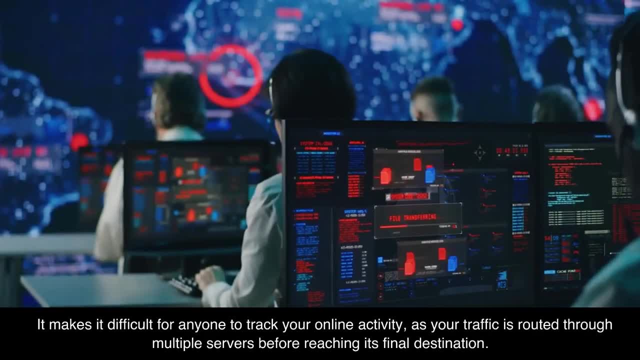 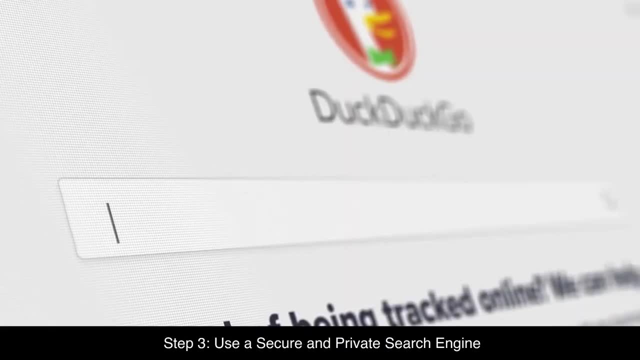 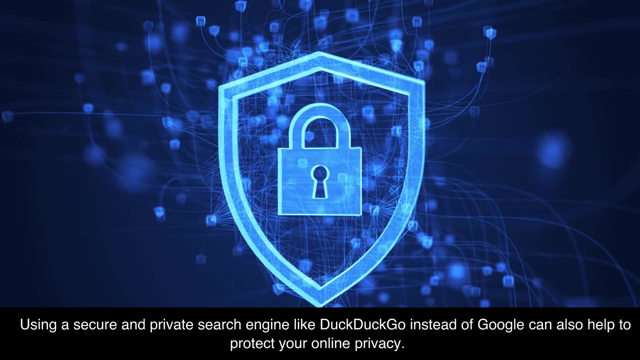 your internet traffic. It makes it difficult for anyone to track your online activity, as your traffic is routed through multiple servers before reaching its final destination. Step 3. Use a Secure and Private Search Engine. Using a secure and private search engine like DuckDuckGo instead of Google can also help to protect your online privacy. DuckDuckGo doesn't. 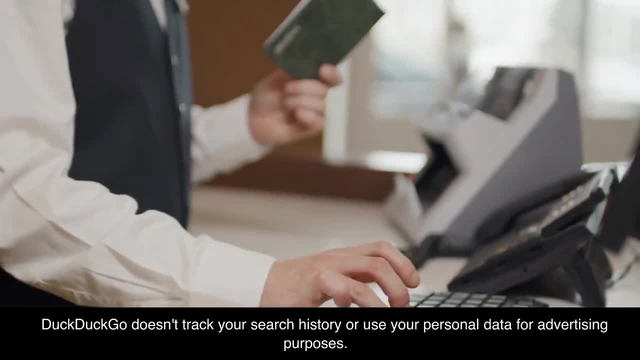 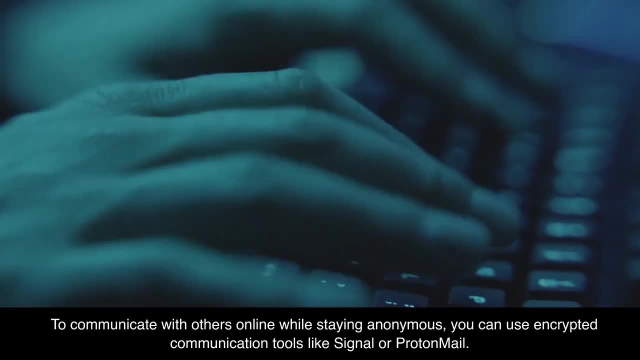 track your search history or use your personal data for advertising purposes. Step 4. Use Encrypted Communication Tools To communicate with others online while staying anonymous. you can use encrypted communication tools like Signal or ProtonMail. These tools use end-to-end encryption. 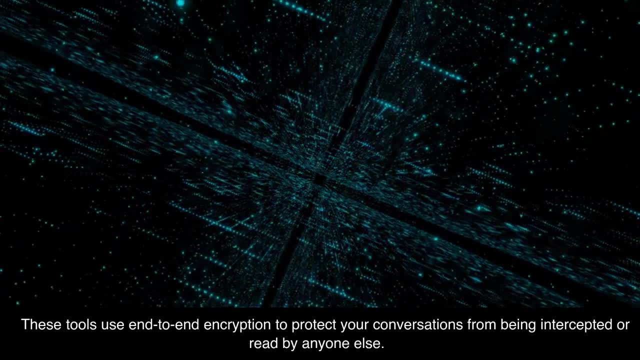 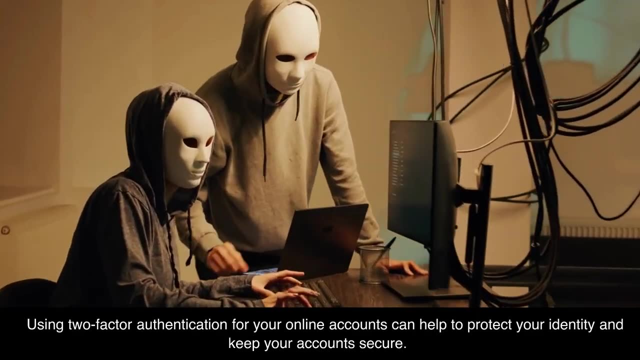 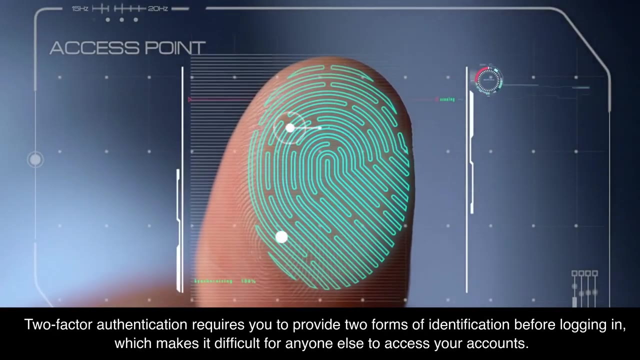 to protect your conversations from being intercepted or read by anyone else. Step 5. Use Two-Factor Authentication. Using two-factor authentication for your online accounts can help to protect your identity and keep your account secure. Two-factor authentication requires you to provide two forms of identification before logging in, which makes it difficult. 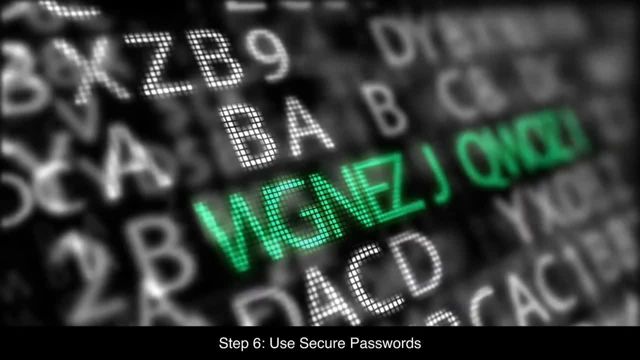 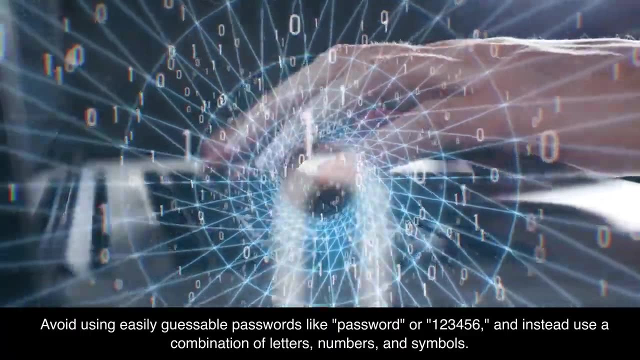 for anyone else to access your accounts. Step 6. Use Secure Passwords. Using secure passwords can also help to protect your online identity. Avoid using easily guessable passwords like password or 123,400 passwords. Step 5. Use Two-Factor Authentication. Using two-factor authentication. 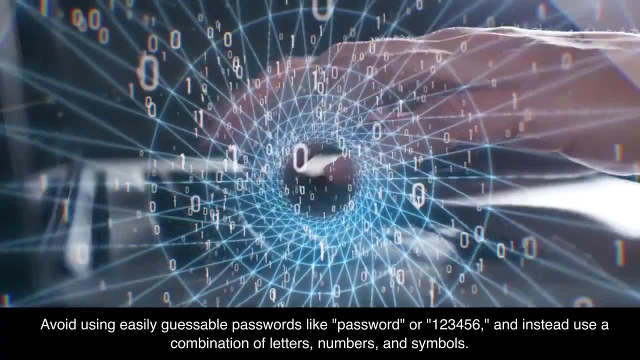 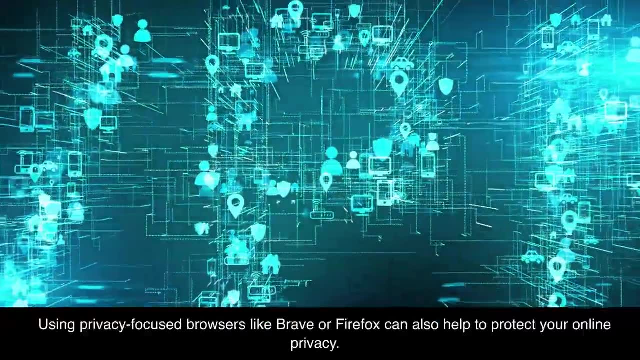 can also help to protect your online privacy. You can also use one-factor authentication to protect your online identity. Step 6. Use Privacy-Focused Browsers. Using privacy-focussed browsers like Brave or Firefox can also help to protect your online privacy. These browsers 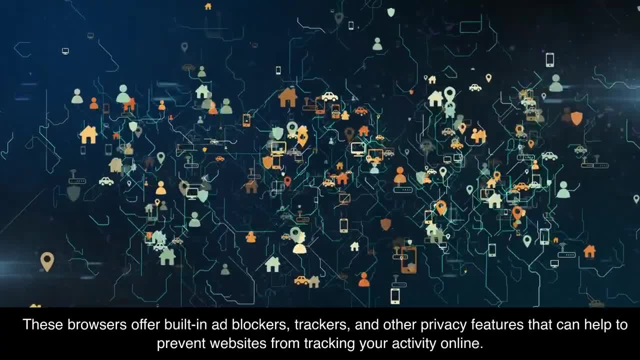 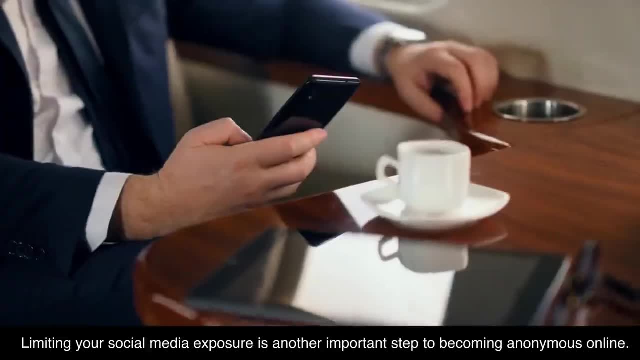 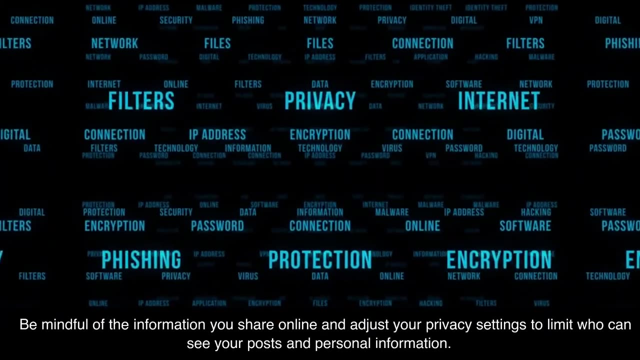 offer built-in ad blockers, trackers and other privacy features that can help to prevent websites from tracking your activity online. Step 8. Limit Your Social Media Exposure. Limiting your social media exposure is another important step to becoming anonymous online information you share online and adjust your privacy settings to limit who can see your 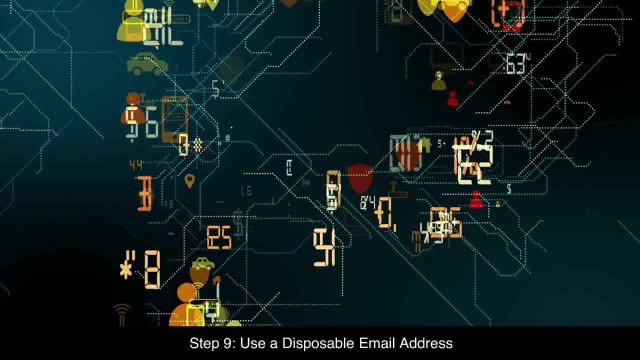 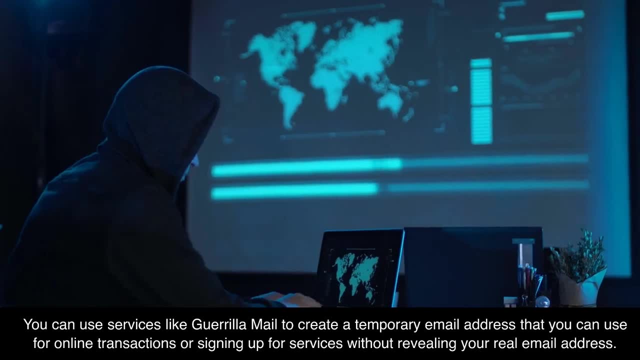 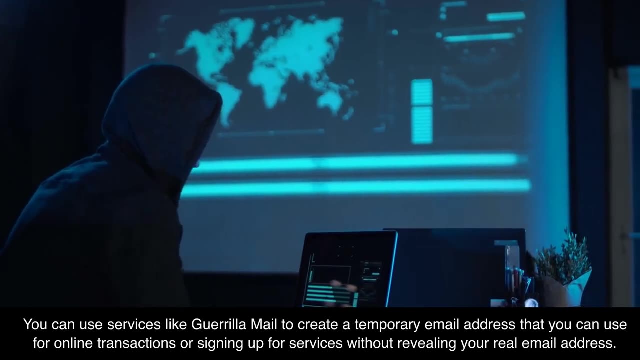 posts and personal information. Step 9. Use a disposable email address. Using a disposable email address can also help to protect your online identity. You can use services like Guerrilla Mail to create a temporary email address that you can use for online transactions or signing up for services without revealing your real email address.